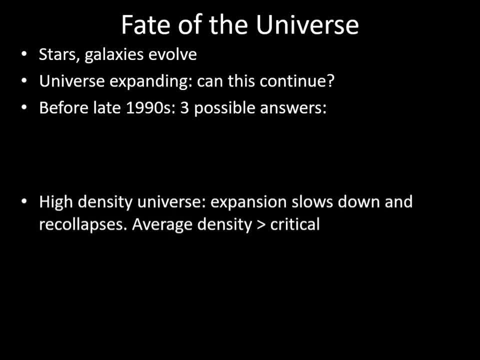 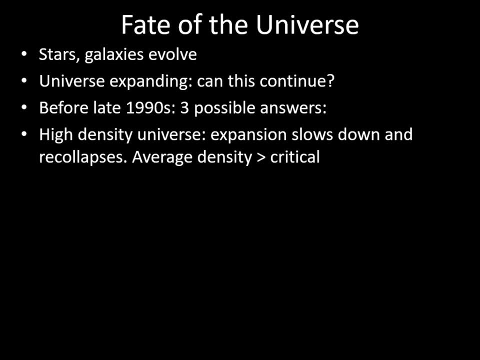 and they were based on the overall average density of the universe. The first option was that the universe would only expand so far, and then gravity would make the expansion stop and reverse itself. This would happen if the average density of matter and dark matter in the universe was larger than a certain value known as the. 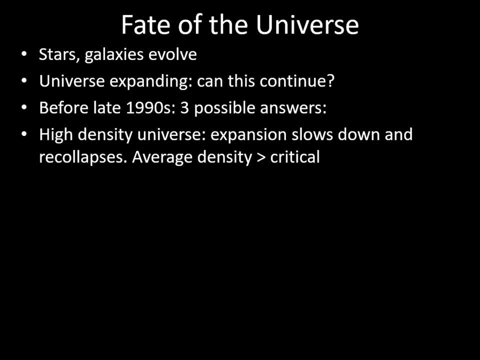 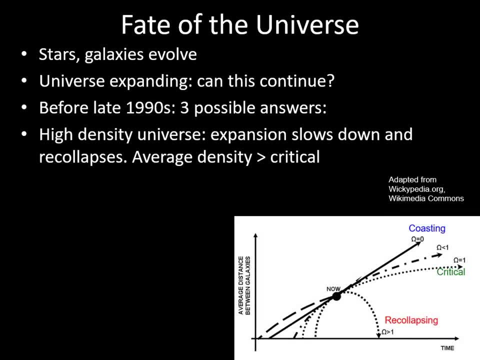 critical density. A universe that expands and then contracts back on itself is known as a re-collapsing universe. On the right we see a diagram showing the relative size of the universe over time, with the re-collapsing universe shown in red. 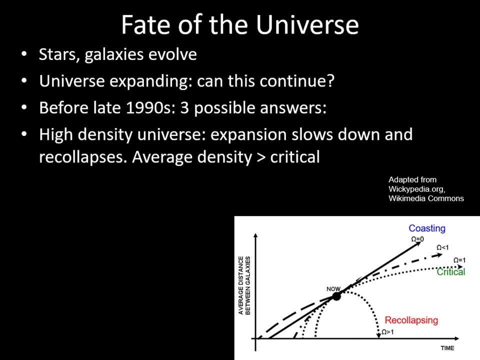 You can think of the re-collapsing universe as the what-goes-up-must-come-down model, In the same way that if you throw a ball up in the air, sooner or later it will fall back to the ground. In this model, the universe starts out flying apart, but sooner or later gravity pulls. 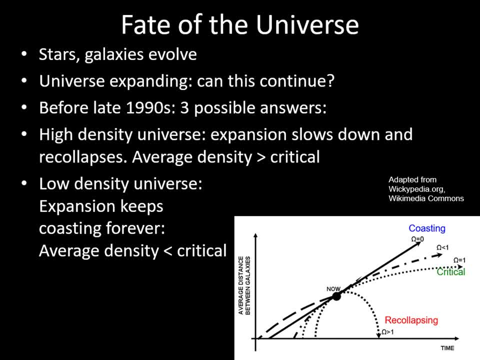 it all back together. The opposite extreme is one in which the density of the universe is less than the critical density. In this case, the expansion keeps going forever. In the figure on the right, this is shown as the coasting universe. It effectively means that the gravity of the 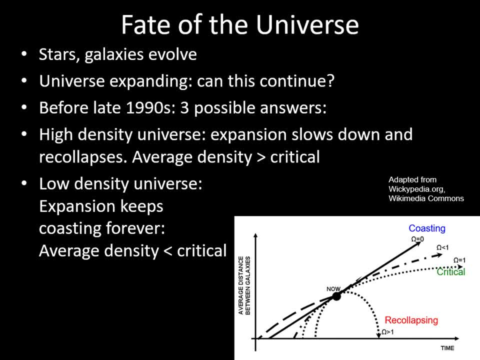 universe is too weak to slow down the expansion. A way to visualize this is by looking at the graph on the right. The graph on the left shows the expansion of the universe. This is to imagine standing on a small asteroid and throwing a ball upward. If the asteroid's gravity is very weak, then the ball won't. 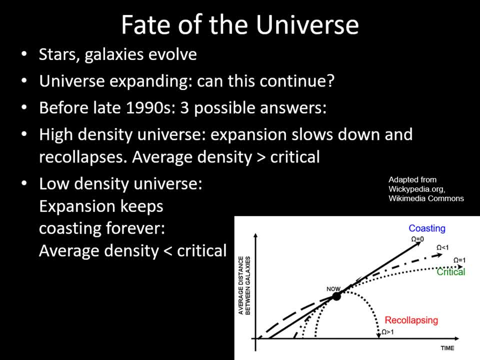 fall back down. Instead, it will keep flying away from the asteroid forever. The last option is called the critical universe. In this case, the universe is exactly at the critical density. The expansion keeps slowing down here, but never quite comes to a stop. 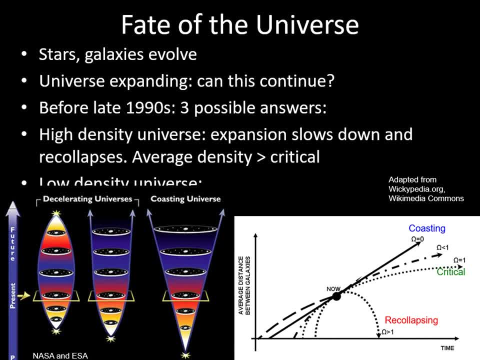 Here's another picture to help you see what's going on. On the left, you see the re-collapsing universe which starts at a point and expands for a while before collapsing back to a point. On the right, we've got the coasting universe that expands outward. 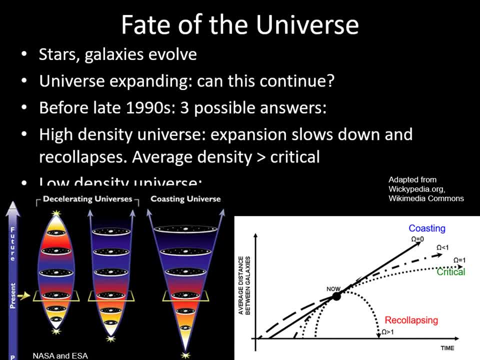 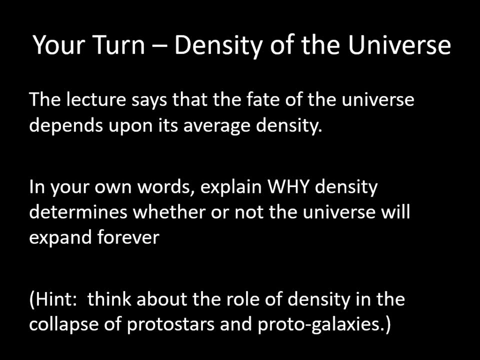 without slowing down significantly at all. Finally, the critical universe is in the middle, expanding at ever slower rates but never quite turning around and re-collapsing. Try explaining in your own words why density is important in determining the fate of the universe. 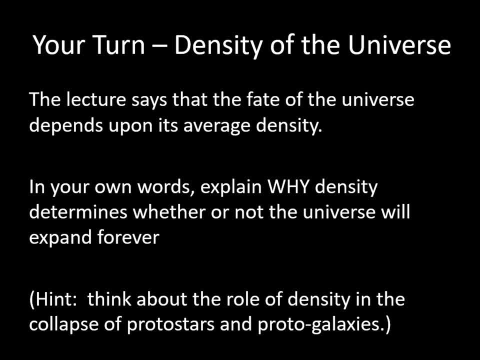 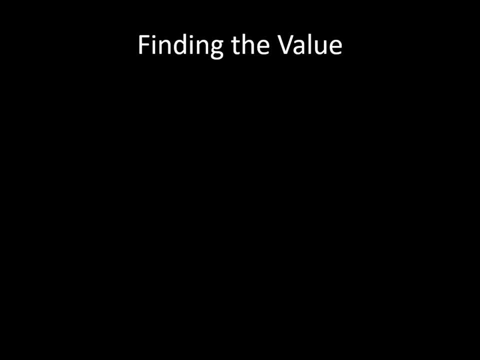 To do this? you might think about other times where we've discussed the role of density in topics like the formation of stars and galaxies. So what kind of a universe do we live in? To find out whether or not the density of the universe is larger, smaller or the same as the critical density, there are two basic 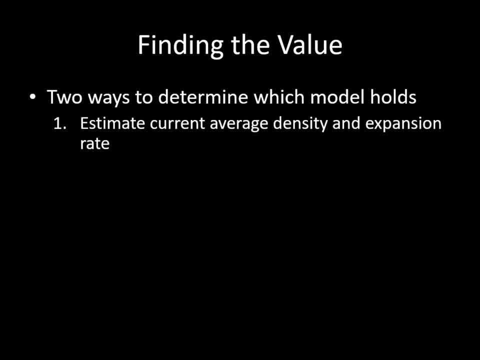 approaches we can try. We estimate the average density of the universe, including all of the dark matter, and compare this with the critical density, which depends on how fast the universe is expanding. In other words, the critical density is tied to the Hubble constant. we saw a couple of 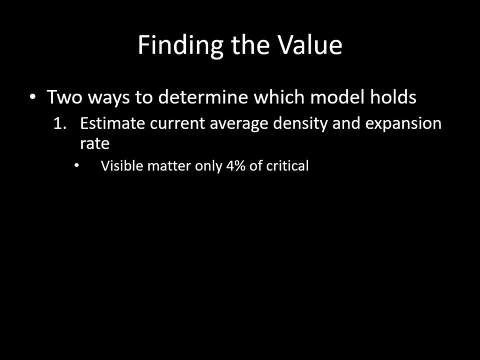 chapters ago. When we do this, we find that the visible matter makes up about 4% of the critical density. When we include in the dark matter, it comes out to 30% of the critical value. This tells us that we are in a coasting universe that will keep expanding forever. However, 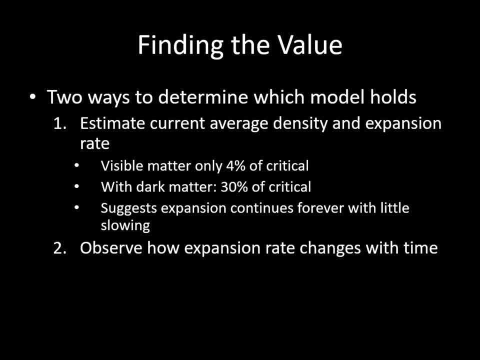 there is another approach, and that is to see how the rate of expansion has changed in the past. To do this, we need both distances and speeds to galaxies that are billions of light years away to see whether they were expanding apart at the same rate. that things. 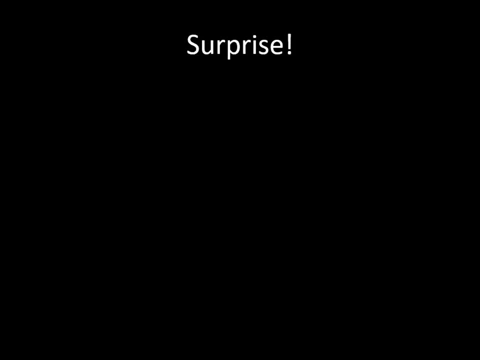 are expanding. now We can measure speeds to distant galaxies easily using redshifts, As we saw earlier. measuring distances is more challenging. We can't use the Hubble law here, because we're trying to test how constant the Hubble constant really is. 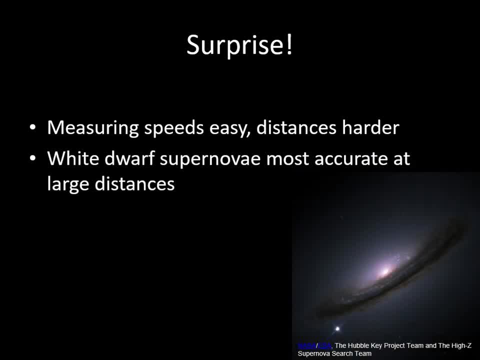 In the 1990s, astronomers began using white dwarf supernovas as an accurate way of measuring distances to very distant galaxies. However, when the supernova distance data came in, it provided a surprise. It didn't match any of the predicted models of the expansion. Instead, it showed that 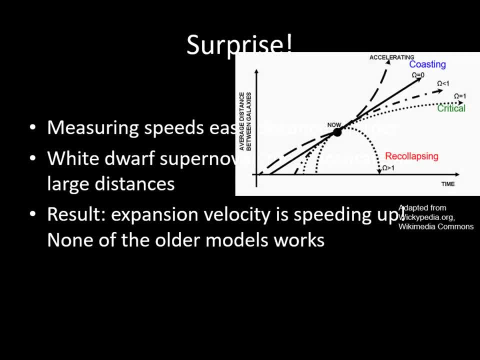 the expansion of the universe has been speeding up rather than coasting or slowing down. This is like throwing a ball up into the air and having it go faster the higher it goes. Since these initial observations, there have been many attempts to find errors in the supernova. 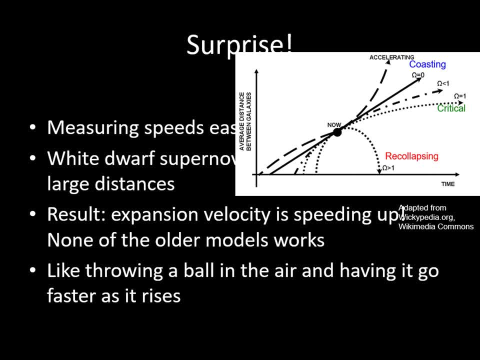 distance measurements, But even with several independent groups working on the problem, it's clear that this acceleration is the most likely one. There are no attempts to find errors in the supernova distance measurements, But even with several independent groups working on the problem, it's clear that this acceleration is the most likely one. 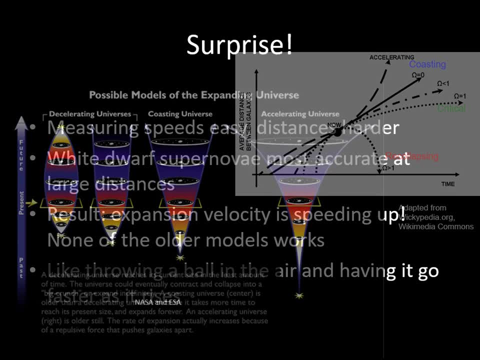 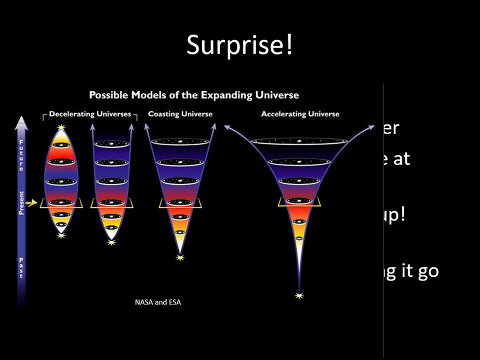 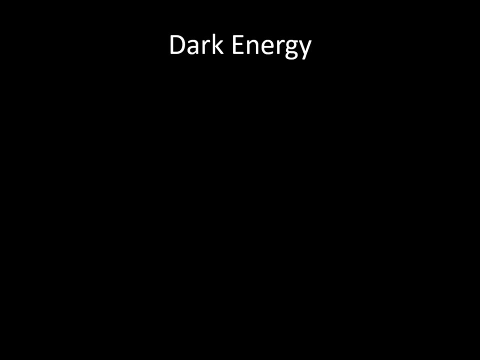 is real. So now we have a fourth model for the expansion, known as the accelerating universe. Exactly what this will mean for the fate of the universe depends a lot on what causes the acceleration to occur. In order for the expansion of the universe to accelerate, there has to be a 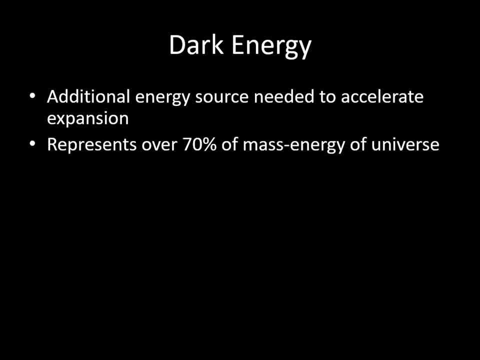 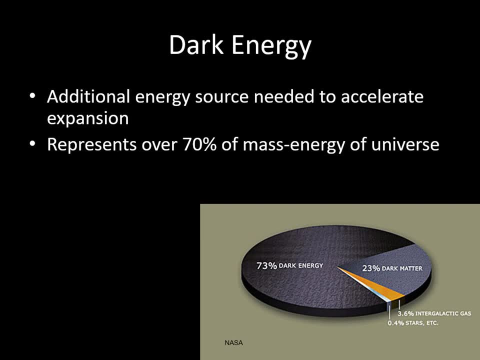 source of energy. There's evidence that this energy would have to represent around 70 percent of the mass energy in the universe, bringing the total up to the critical density. The name we give to this mysterious energy is dark energy. There are several ideas about what 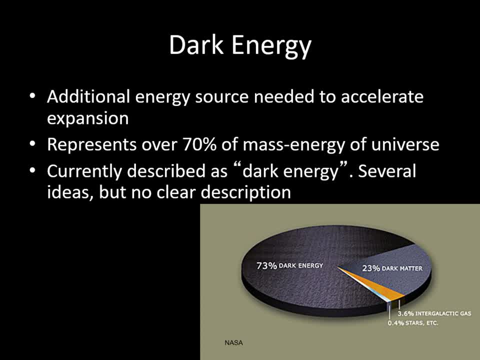 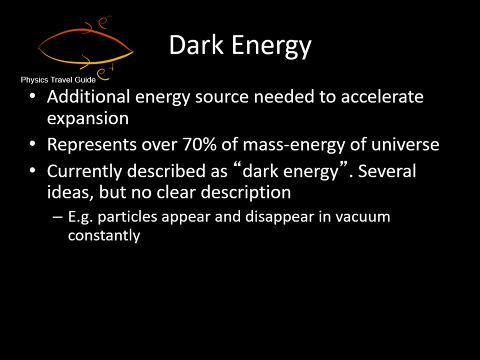 dark energy could be, but no well-tested model for it yet. One set of approaches to this involves something known as the Casimir effect. Particle physics models predict that incredibly short-lived virtual particles should be applied to the universe, Appearing and disappearing all of the time everywhere in the universe, even in complete. 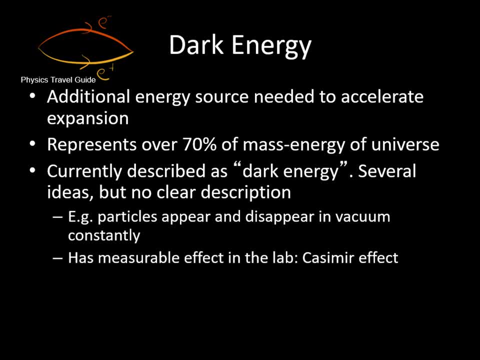 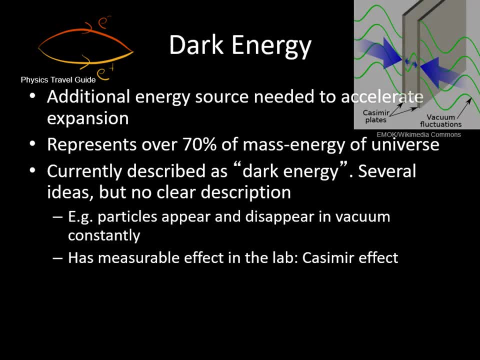 vacuum. these particles have a measurable effect in the lab, known as the Casimir effect. The Casimir effect is measured when we bring two parallel plates very close to each other. We find that there is a force pulling the two plates together because the density of the virtual 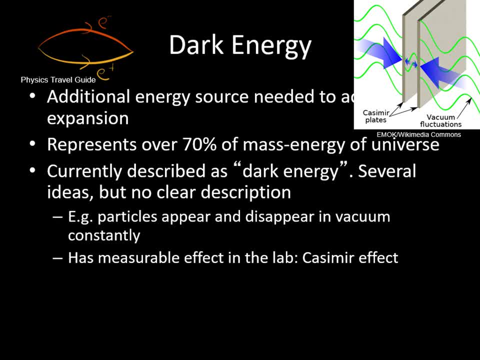 particles outside the plates is larger than the density between them. This effect has been measured for many years and it is used to calibrate models of how these virtual particles behave. Unfortunately, the simple calculations of the energies involved in virtual particles come up with values many orders of magnitude larger than that observed for dark energy. 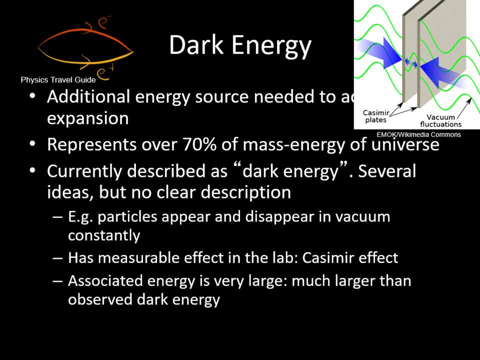 Either something is causing only a small part of the Casimir effect energy to play a role in the experience of the future energy and, in their turn, a На-dense force that works on the quasigal energy, which would mean minus one percent for the Virtual Arts at the time. 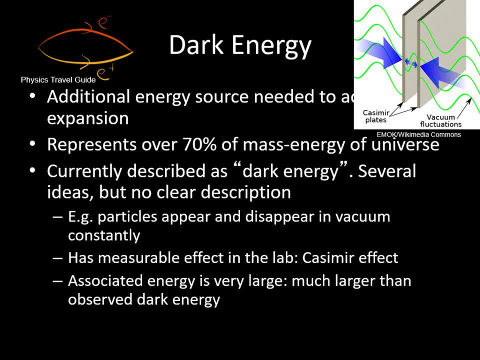 At the same time, the light energy is more forgiveable and it gets a longer period of the expansion of the universe. or there is some other effect entirely behind the dark energy. At the moment, this is the cutting edge of modern physics, so it may be some.